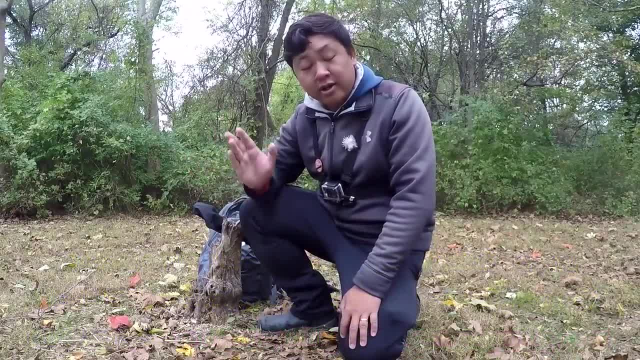 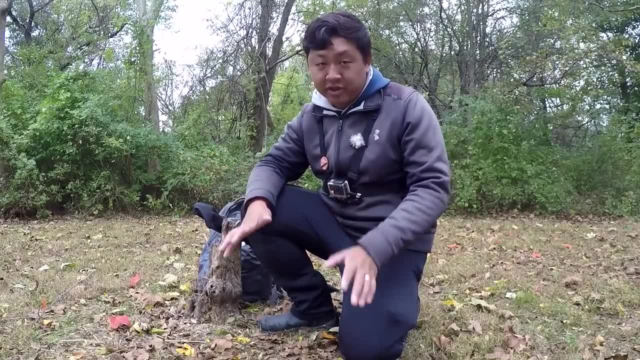 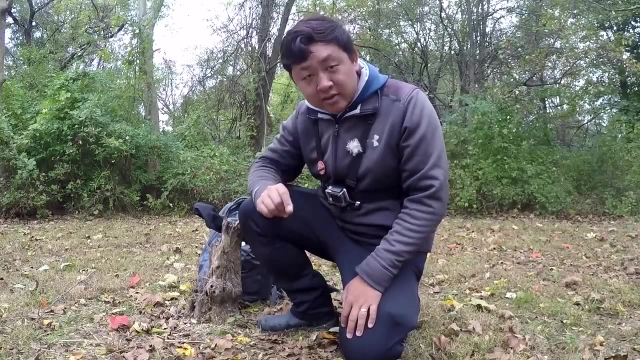 we were targeting those species. we had no idea what they were. we were not targeting them per se, right, They came up by accident. so they are not supposed to be targeted in the state of Pennsylvania. okay, Because they are endangered also if any of you ever comes into contact with those species in this state. this is just a disclaimer. 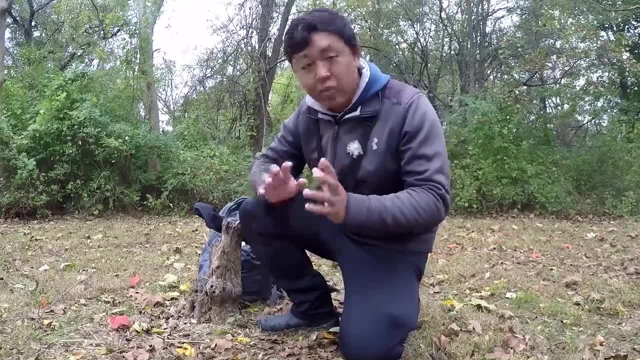 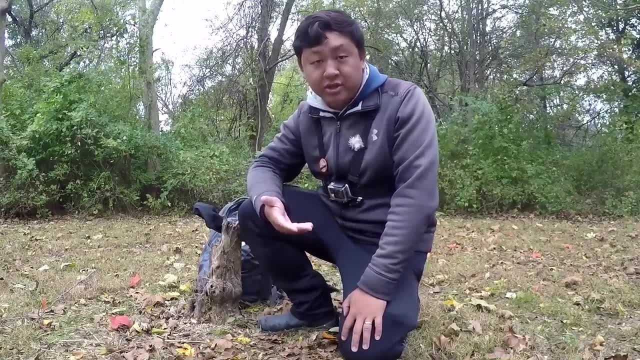 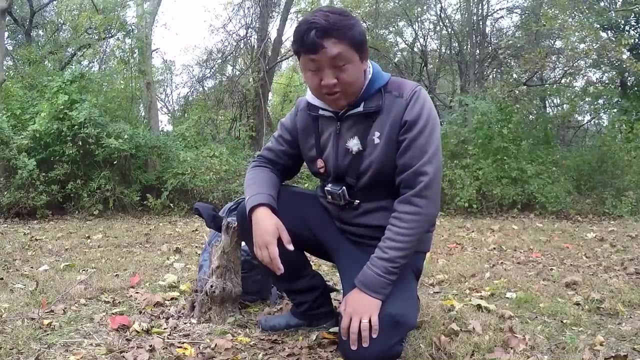 make sure that you take very, very good care of them and release them right away. okay, They may be micro-species, they may be shiners, but they are endangered. Their population is in decline. okay, Their native ranges, year by year, is getting smaller and smaller and smaller. Anyways, I did catch all those wonderful species in the Poconos, but I am kind of still of a failure when it comes to my home waters. right, It is the fall trout season and I have yet to catch a fall stock trout here in Philadelphia County, which is why I came to the Penny Pack today. 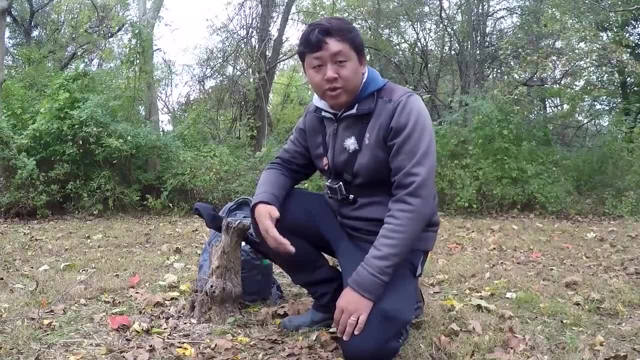 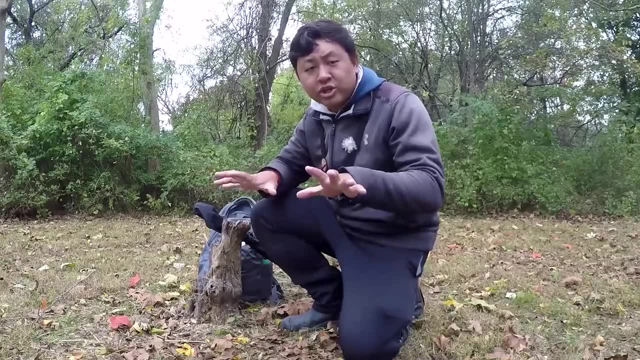 My main objective is just really to land a trout and bring it home so that a creeper can and I can have it for dinner, right? So you know what? Let's go to the creek first and let's check the conditions and we are going to get the fishing started. 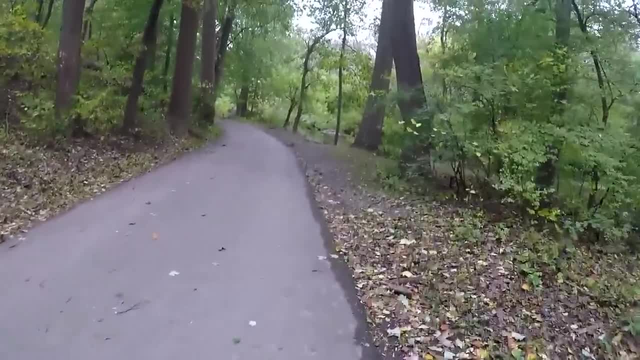 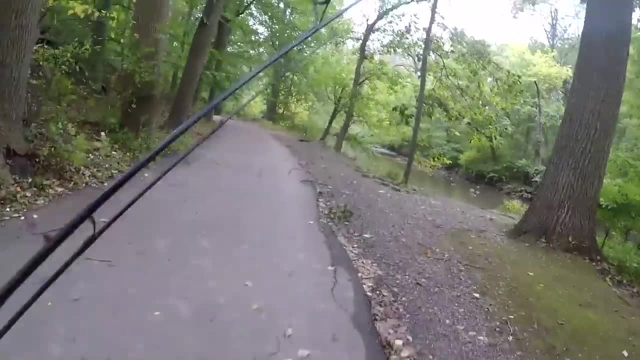 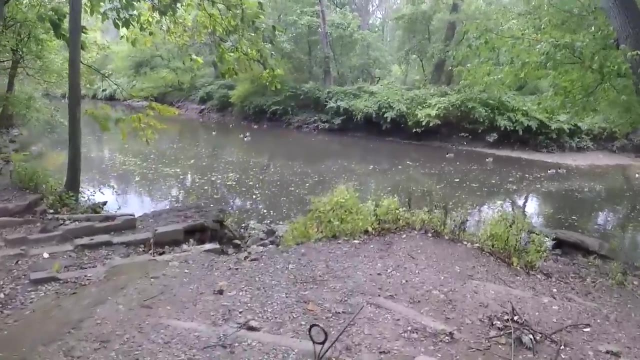 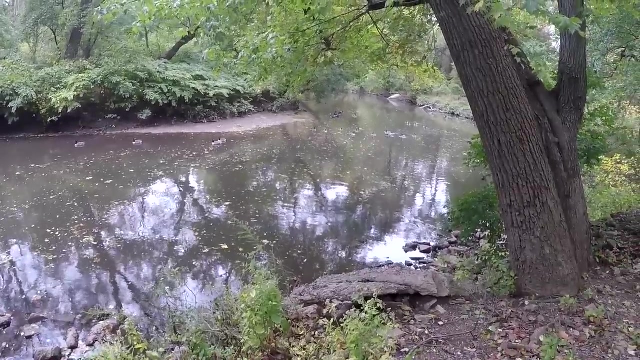 Ladies and gentlemen, this is the moment of the truth. We actually had some pretty heavy rain yesterday around the area, so until this morning the creek was like chocolate milk. Let's see how the creek is looking Right now. Yeah, the flow is still a little bit higher than usual. 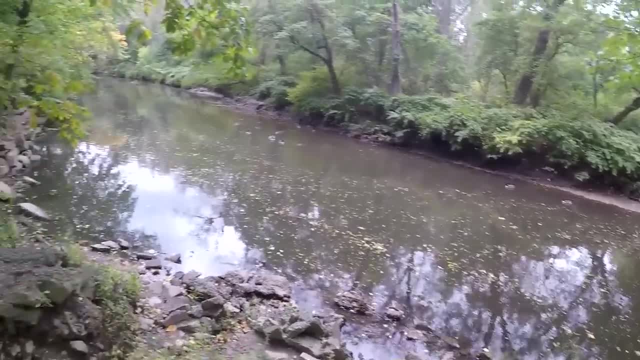 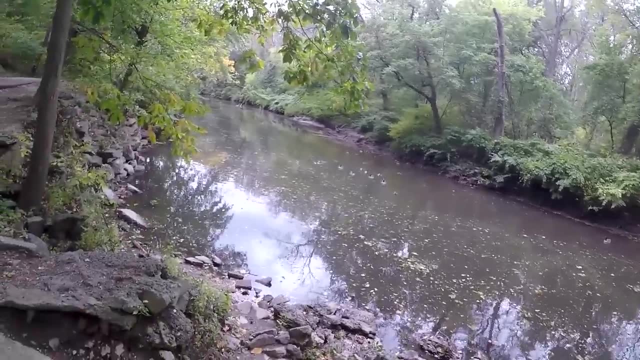 We got the usual amount of geese over here, which is not good. I think I could potentially throw a power bait in there and try to get things done quickly, Or maybe get started with a spinner- although with a spinner- look at all these- leaves right. 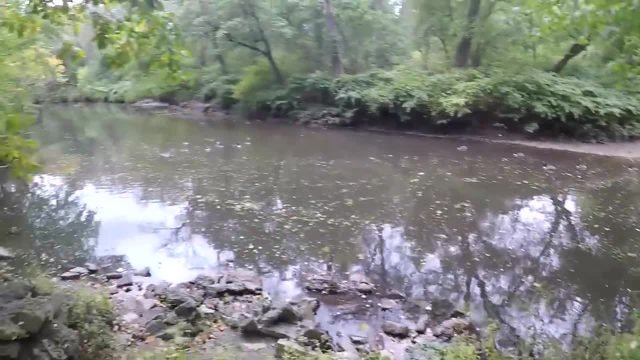 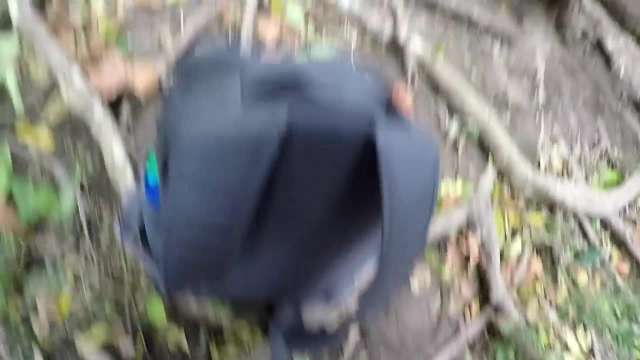 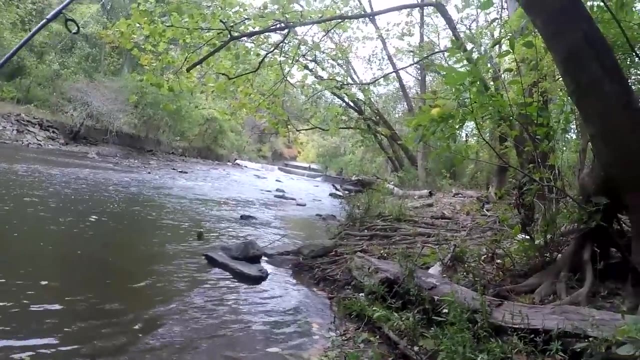 It would make things very complicated. Alright, let me get my stuff ready and let's go catch some fish for dinner. As always, everyone is hitting the dam. I never really understood why everyone loves that dam so much. We got like four people at the dam. 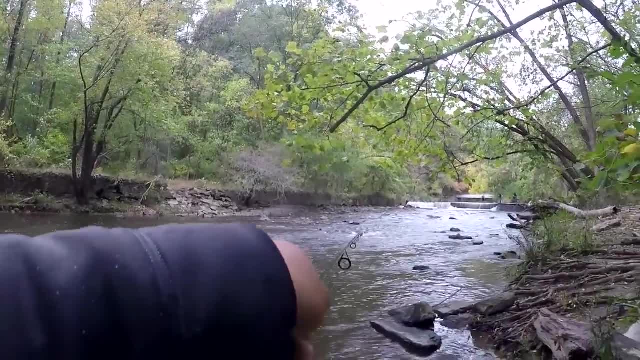 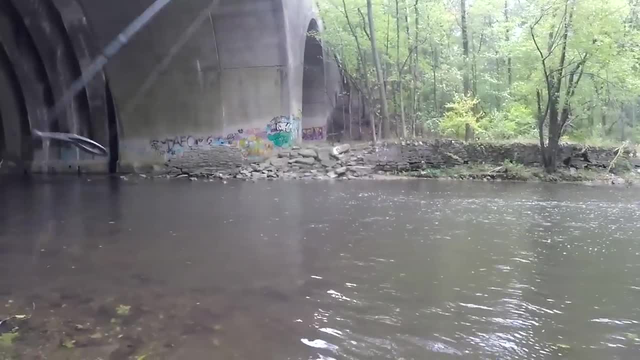 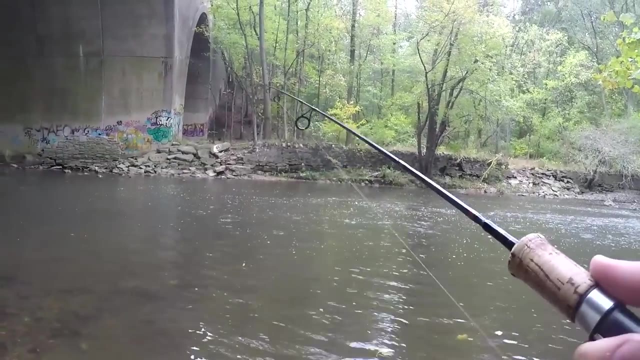 But look at this little spot over here. Look how juicy this little spot is. right, You got the shallow place over there that kind of turns into a flow over here that is a little bit deeper. I'm going to run my Thomas, my trusted Thomas, one six of an ounce inline spinner to see if anything shows up around this area. 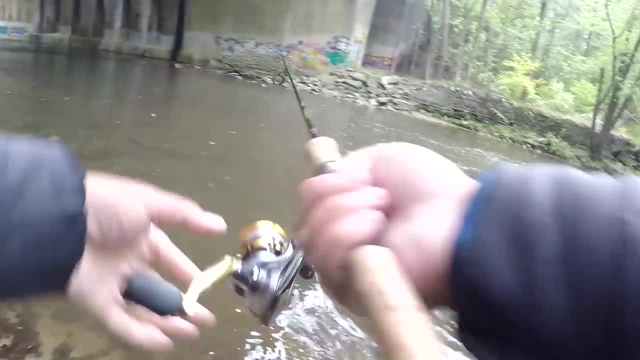 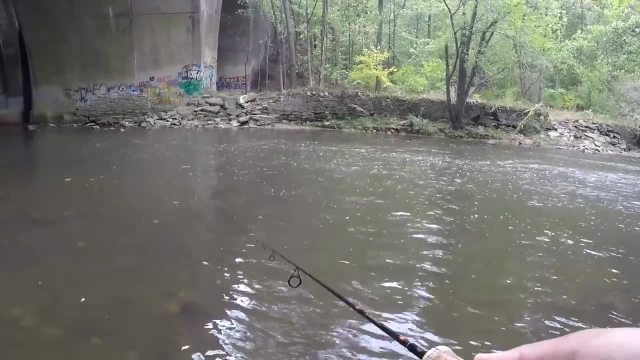 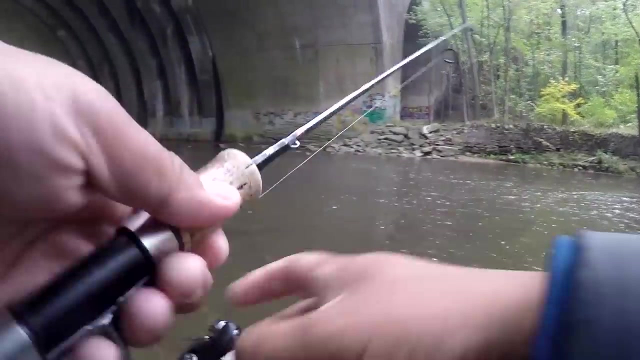 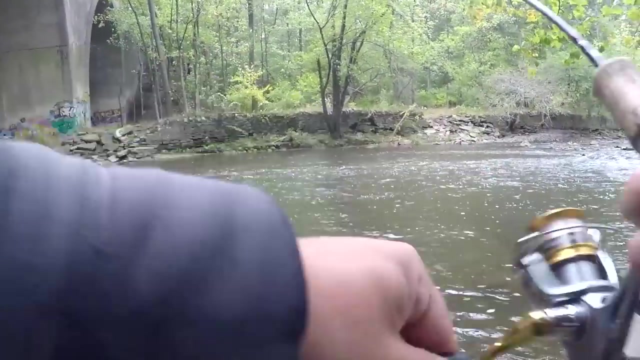 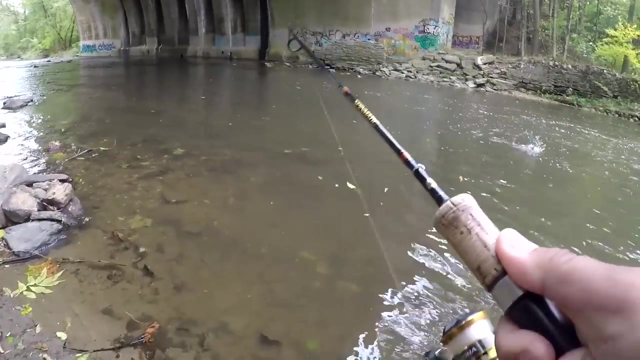 It should be crazy. good for spinners man. Come on, There's one. There's one Spinner man. This is good for spinners. I just knew it. This whole area looks so juicy. You know what I'm saying. 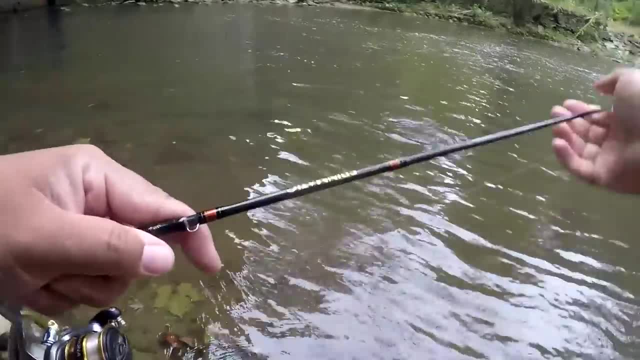 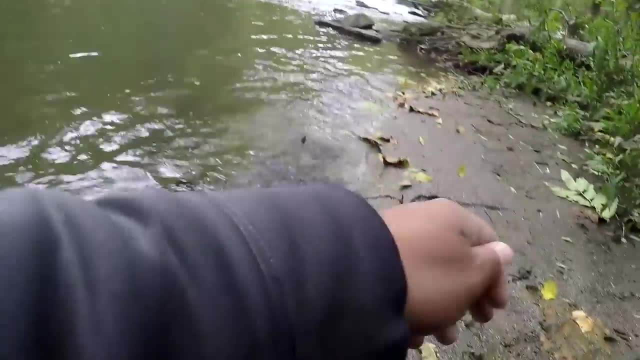 There's a nice size one, too Beautiful. Let's see what we got over here. It's a brown, Holy moly, It is a brown. It's not even a rainbow. It's the Salmo. It's the Salmo, Truta. 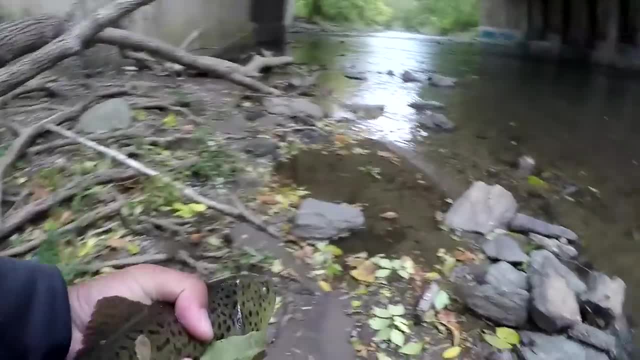 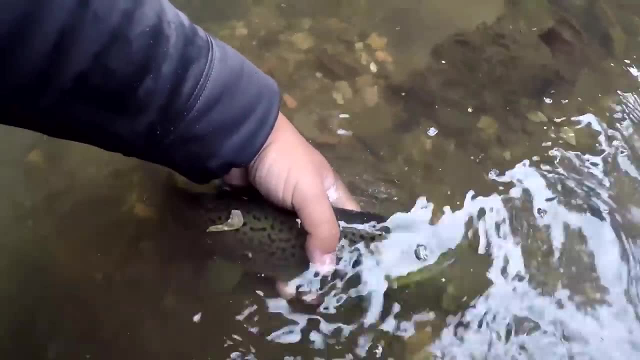 Nice size, brown too Beautiful. Okay, that is pretty not cool. First fish of the day actually turned out to be A brown trout. I kept it outside of the water for a little bit, So I don't know if this fowl is going to be okay or not. 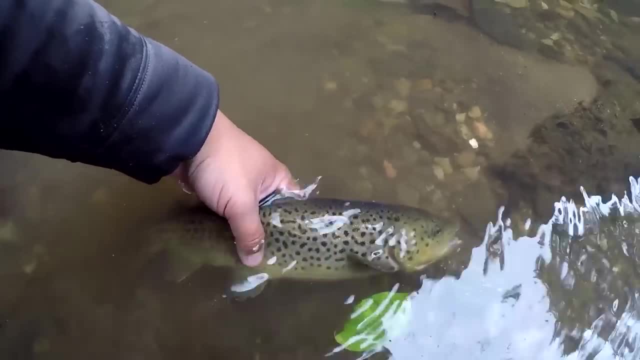 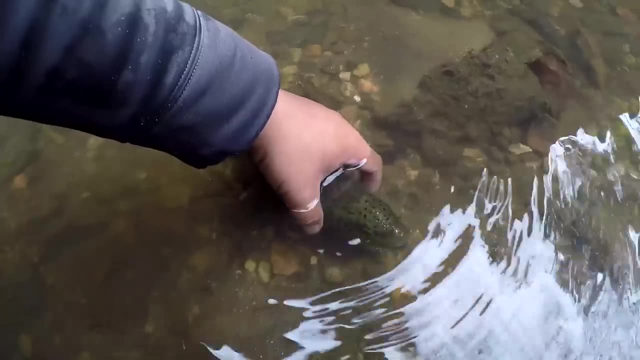 I certainly hope so, But if not, this is a catch and take fishery, So I'll gladly take this brown trout home to eat. It is looking a little bit weak. I think this one was stocked here by accident, though, Because I'm telling you they're not supposed to stock brown trouts here for the fall. 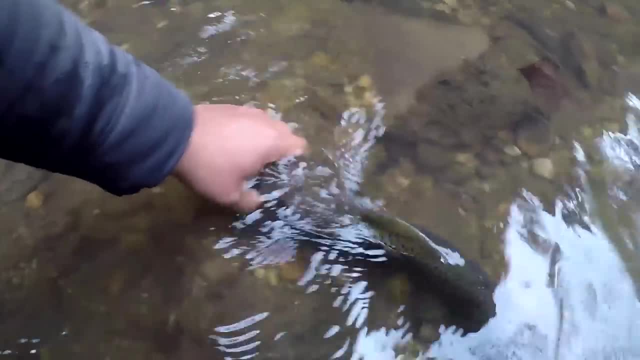 So yeah, I think this one is going to be dinner, man, This trout. Oh wait, wait, wait, wait, wait, wait, wait, No, no, no, no, That one's good to go, Good to go. 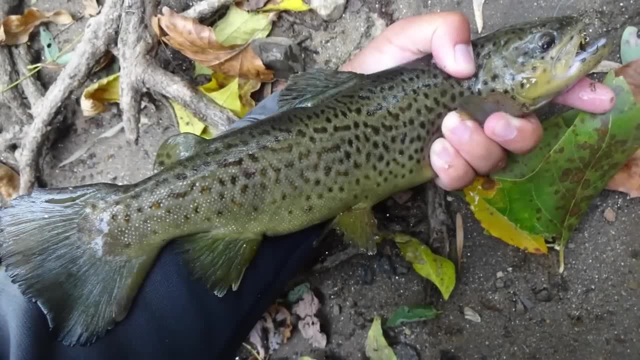 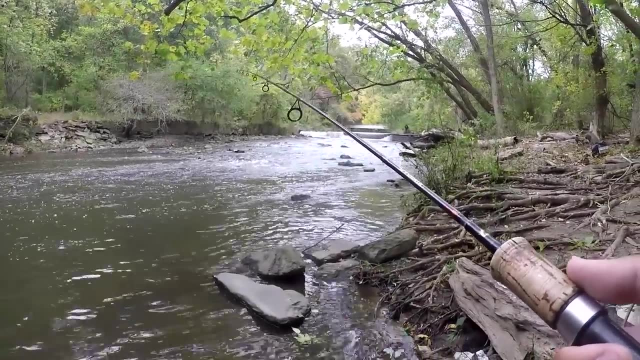 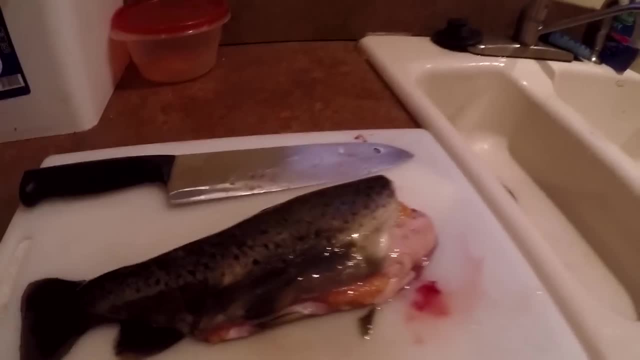 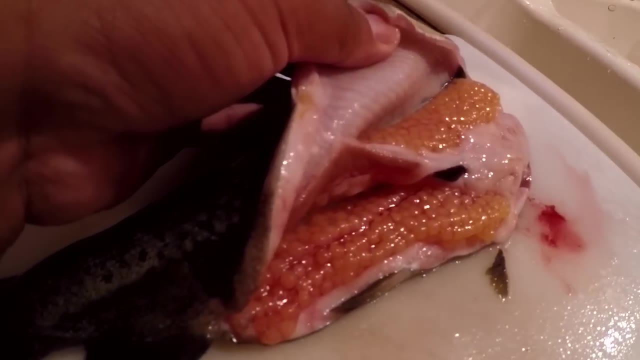 Yeah, it's not bad, So rate it 0 to 10.. How much would you say? This is going to be our dinner, by the way, 7.. 7 out of 10?? Look, coming from Creeper Kid, that's a high rating, okay. 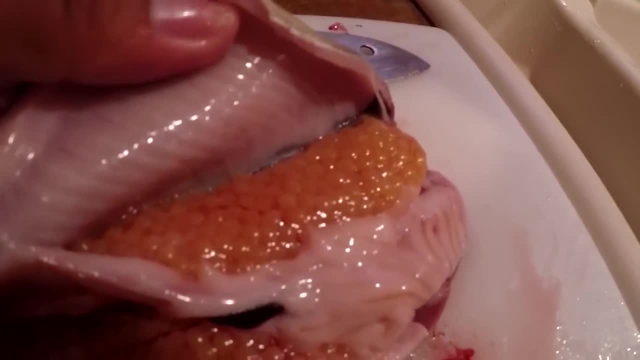 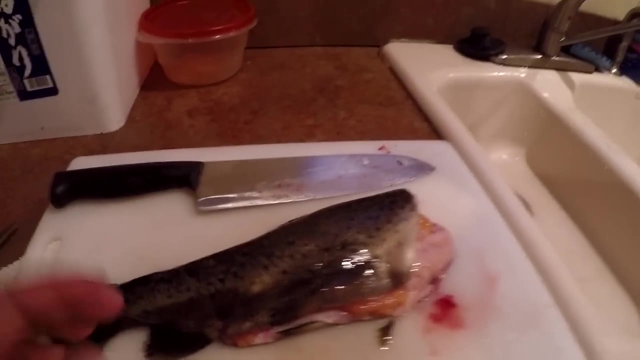 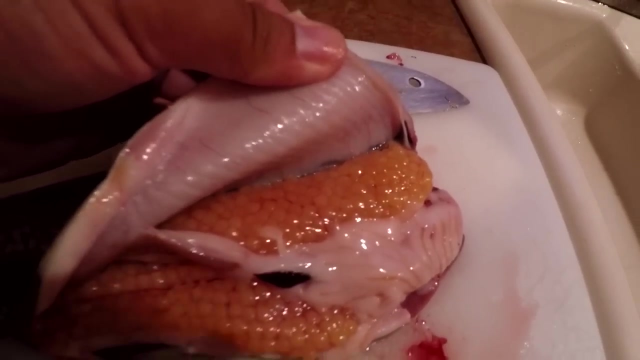 Because the only thing that he raised above 9 is what Steak, right, Um, I guess? Anyways, folks, this is it for this video. I hope you guys enjoyed the trout. catch and cook Fried trout here. I got some other stuff that I have to cook for Creeper Kid. 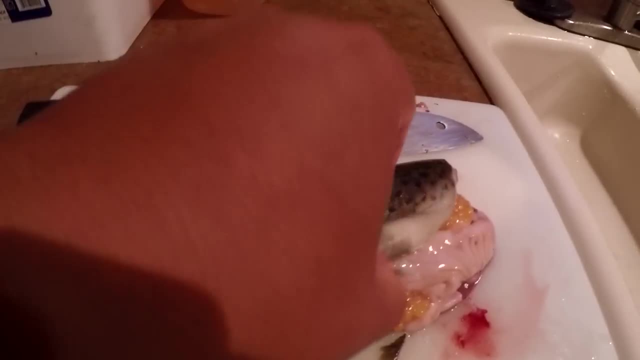 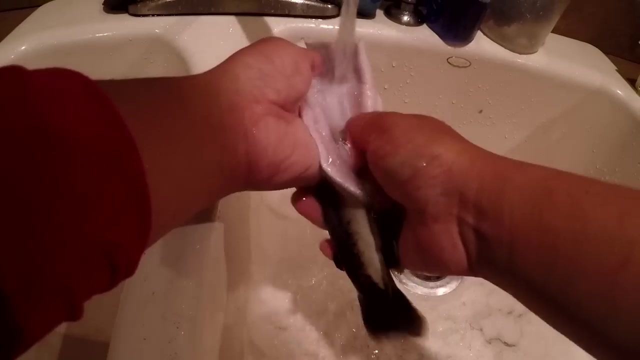 We're not going to have Only the trout for dinner, right? So I'm going to get to cooking. Thank you very much for watching. You want to say anything to YouTube before I turn it off? No, All right, I'll see you guys next time. 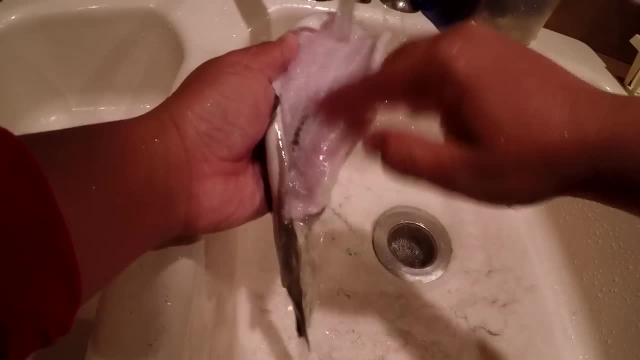 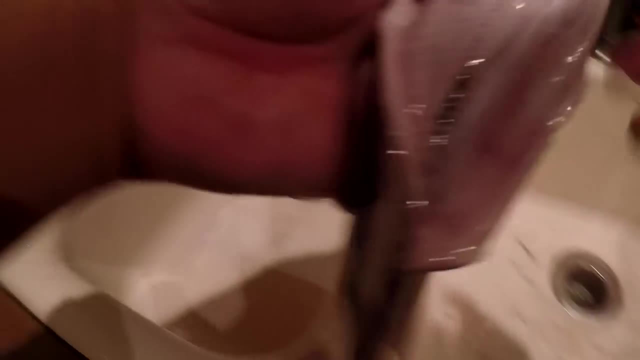 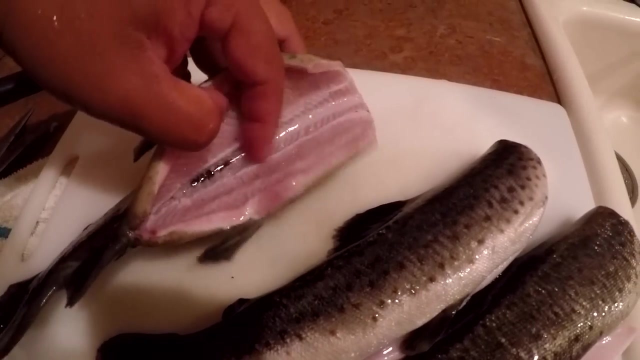 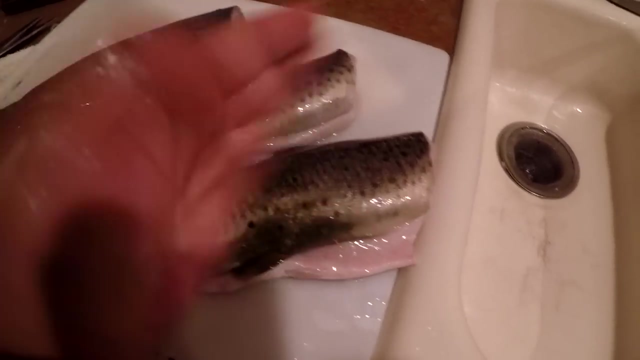 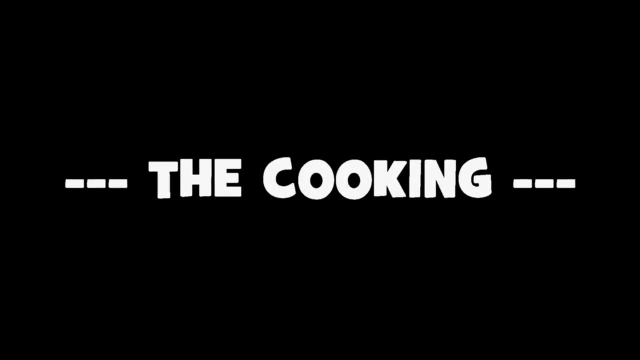 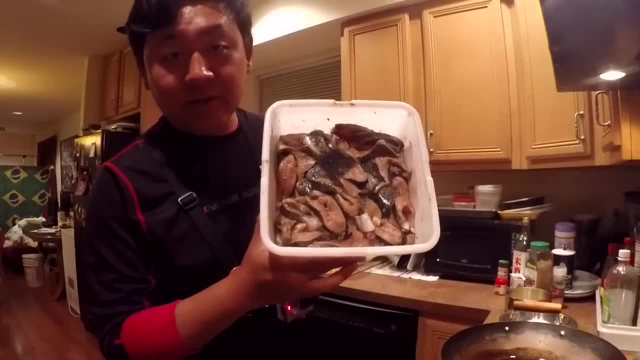 Bye, Bye, Bye, Bye, Bye, Bye, Bye.